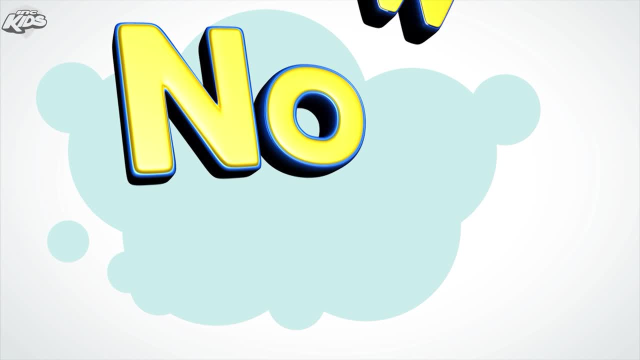 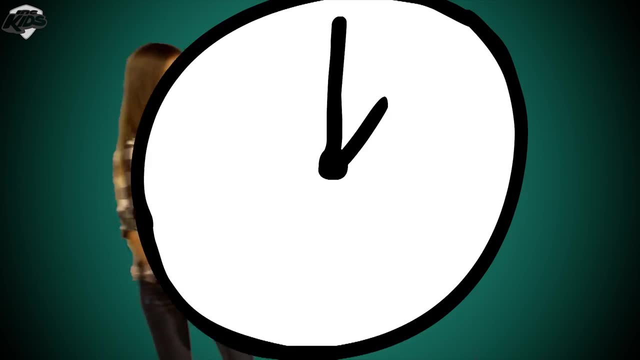 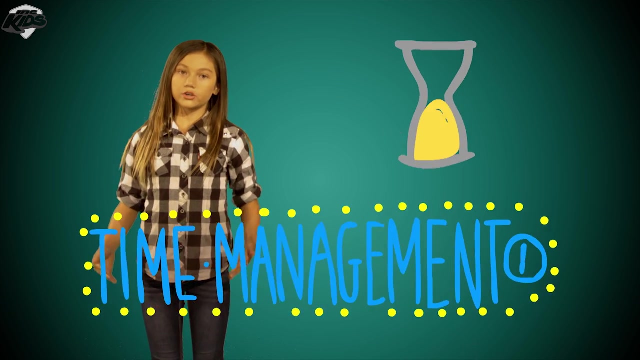 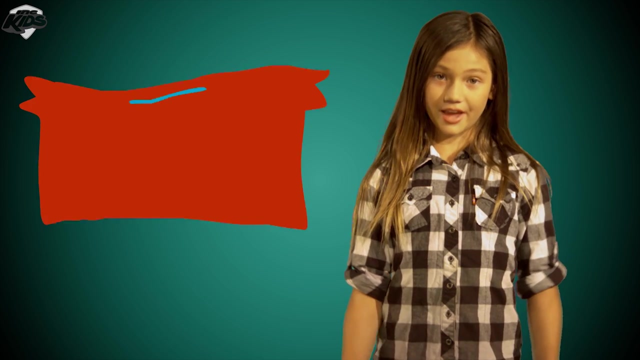 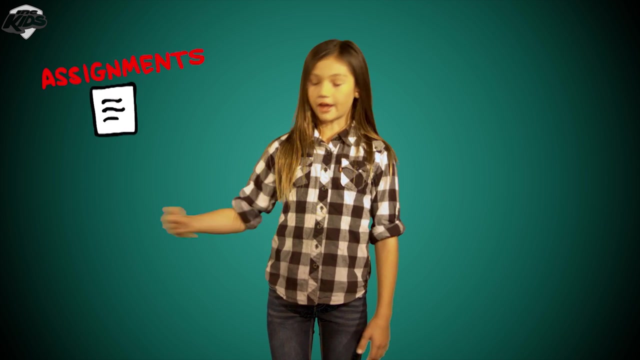 Time management. Time management means organizing your schedule so you get things done without feeling too overwhelmed or stressed out. Here are some tips for time management: Use a day planner or calendar. Write down assignments, tests, meetings, practices and important events so you won't forget. 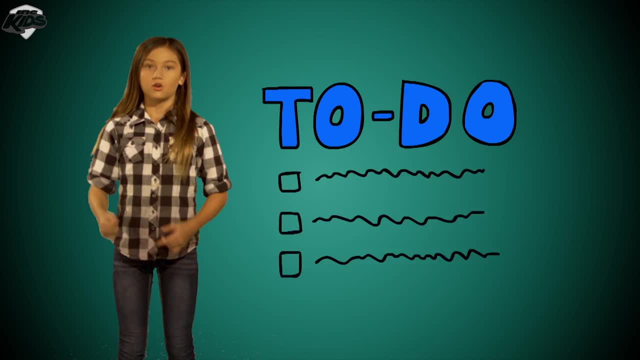 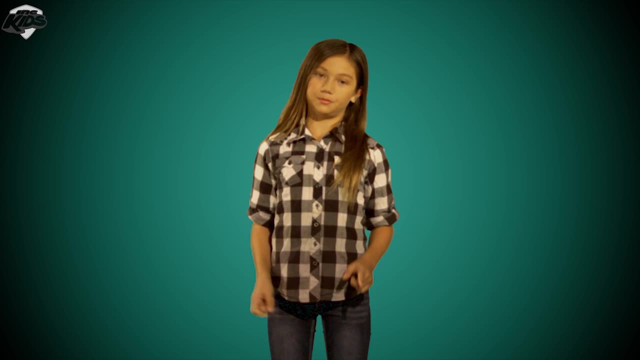 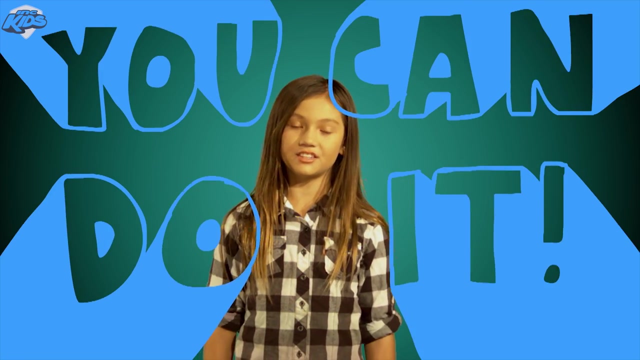 about them. Make a to-do list. Write all your assignments and tasks down and check them off as you complete them. Include deadlines or when they need to be done. Don't procrastinate. If you can get it done now, do it. Try not to leave things until the last minute. 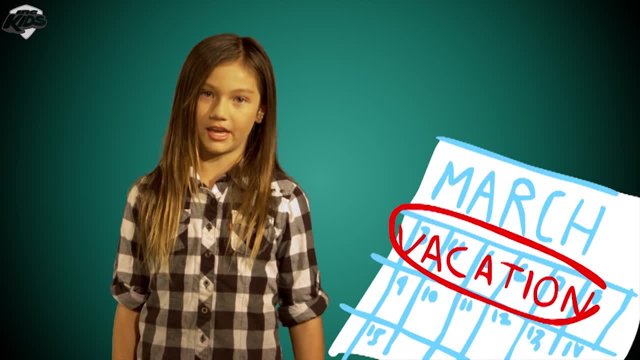 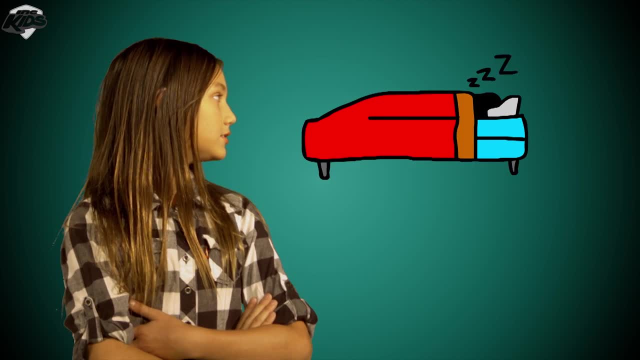 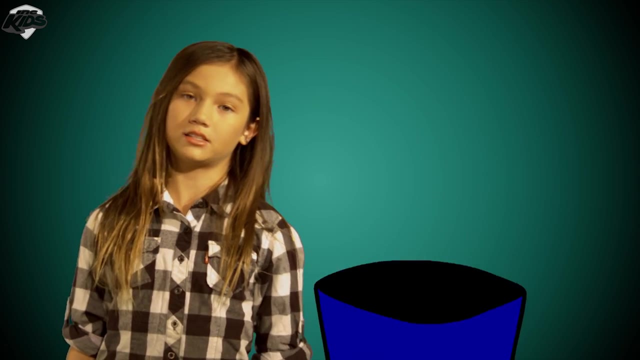 Plan ahead. If you are going on vacation the same day you have an assignment due, make plans to finish it and turn it in early. Use your time wisely. Don't let time get wasted. Use free time between activities. Tackle your reading assignment on the bus, ride to school. 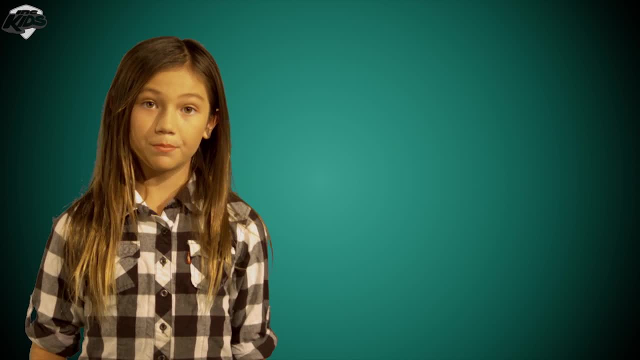 or to a sports competition. If you are busy after school, try to find time to complete work during the school day, For example. if you have a lot of work to do, try to find time to complete your work during the school day, For example. 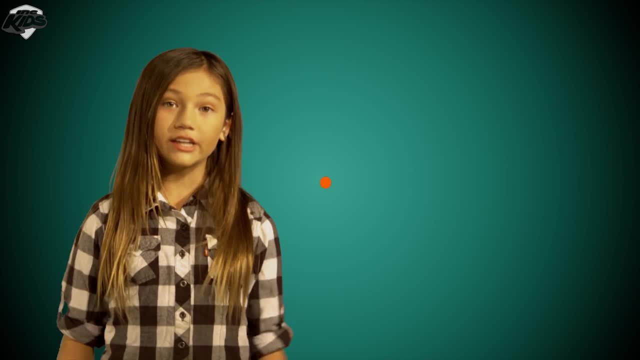 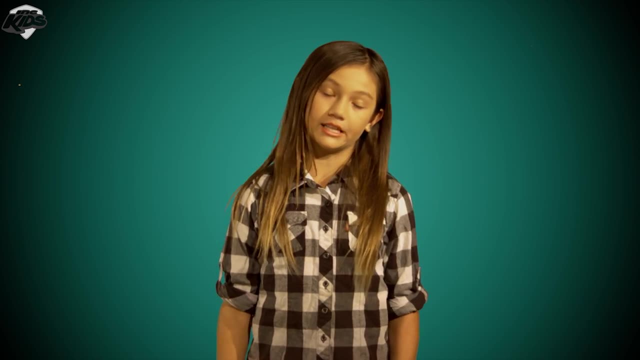 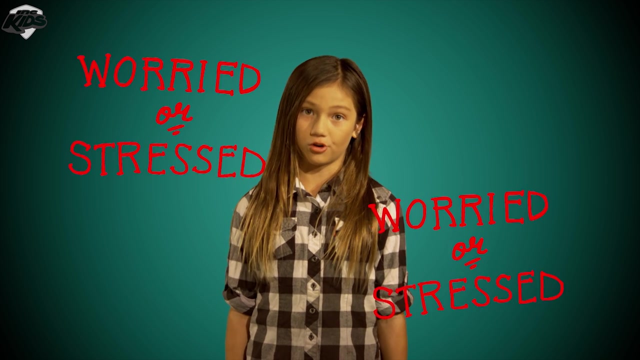 the result might come out during the home run or study hall. It's great to be involved in different afterschool activities, but if you feel rundown, it might be time to let some things go. Pray, Trust that God will help you succeed. You won't be worried or stressed. 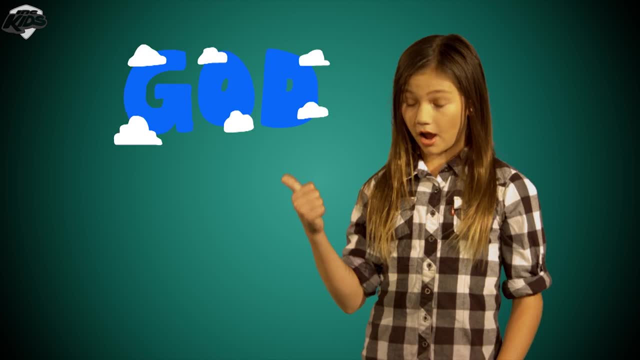 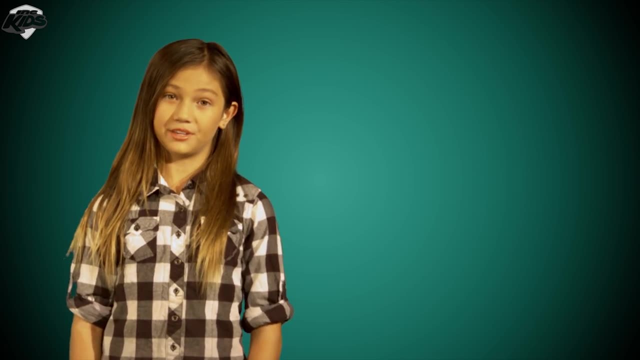 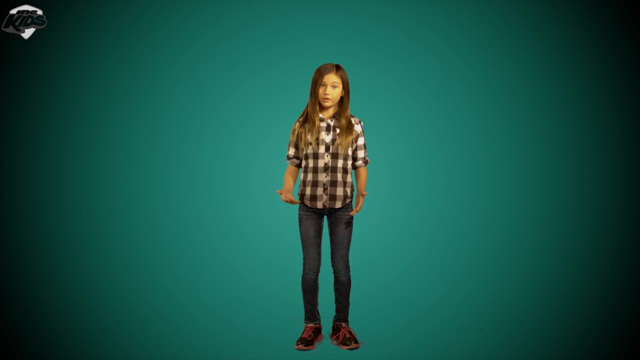 Prioritize. Our order of priorities should be God, family, school and then friends. Attend the worship service should be the most important event in our lives, So write it in your calendar and to-do lists When you get home from school. 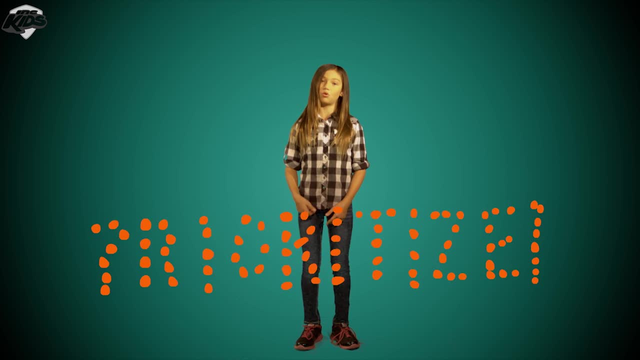 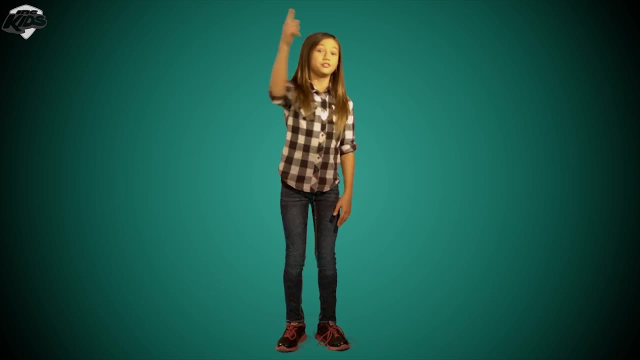 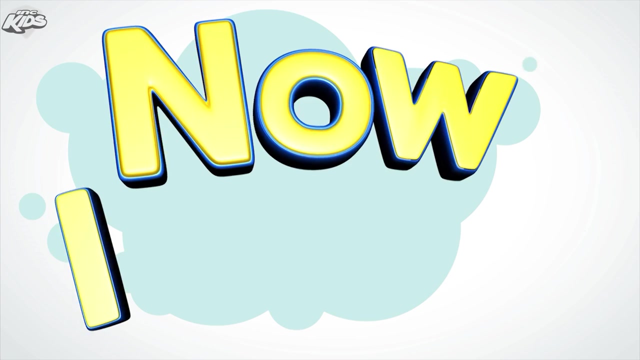 while your homework is fresh on your mind, it is best to do all of it before you hang out with your friends. Manage your time before time manages you. What are some of your tips for time management? Subtitles by the Amaraorg community.